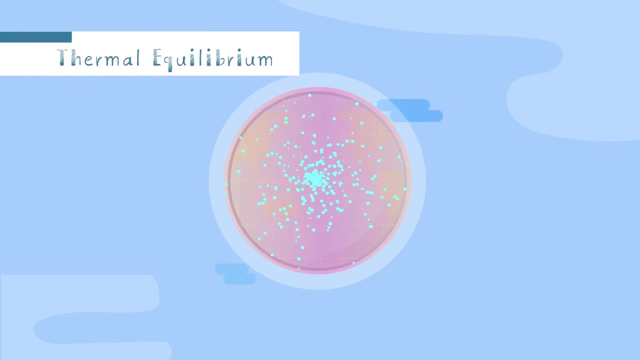 thermal equilibrium. So then, why and how does atmospheric general circulation occur? In order to understand atmospheric general circulation, we first need to properly grasp the concept of latitude. Let's place a protractor on the globe. To measure angles using a protractor first. 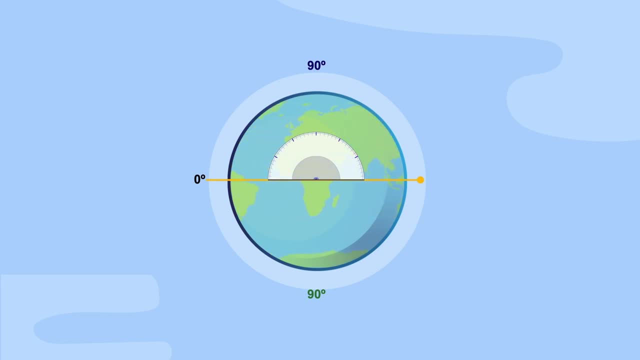 you need to locate the horizontal line on the protractor that indicates zero degrees, since this line is used as a reference for measuring all angles On. this line is a reference for measuring all angles On. this line is a reference for measuring all angles On. 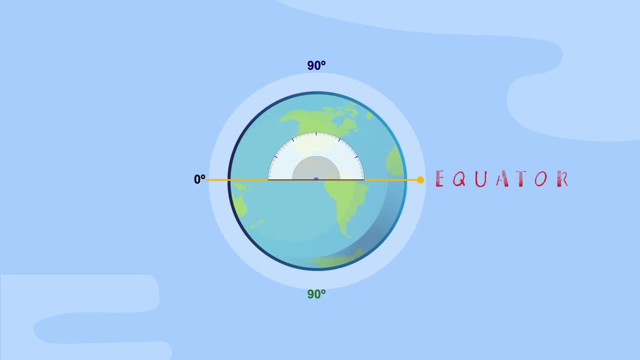 the globe. the horizontal line is at the equator. The earth is divided at the equator into northern and southern hemispheres. The angles 30 degrees, 60 degrees and 90 degrees from the equator are called degrees of latitude. The Sun. 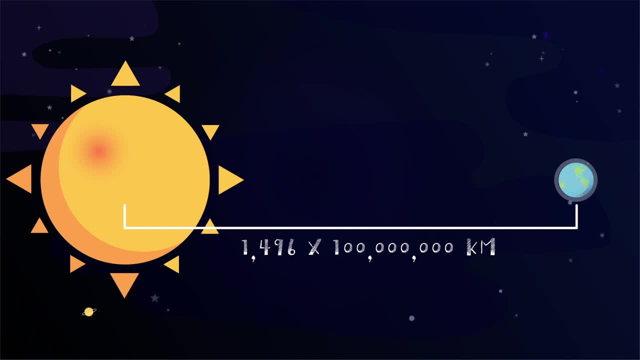 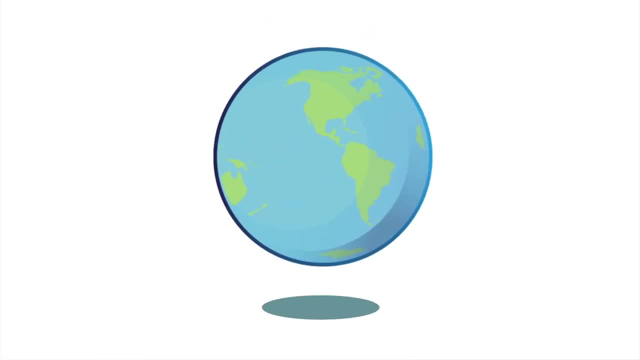 is very far away from the earth Because the earth is so small compared to the Sun. sunlight hits the earth in horizontal lines. Near the equator, the rays of the Sun are more perpendicular to the ground, While at high latitudes, the Sun's rays reach the ground at an angle. This means that the 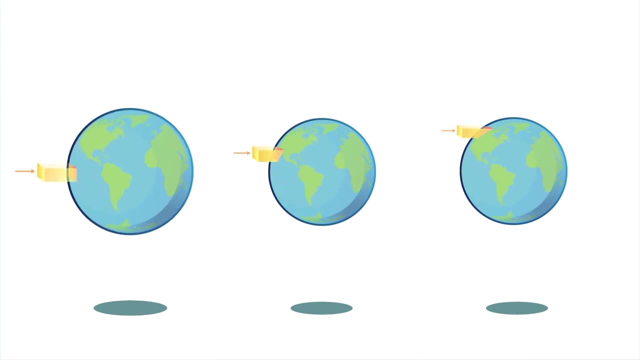 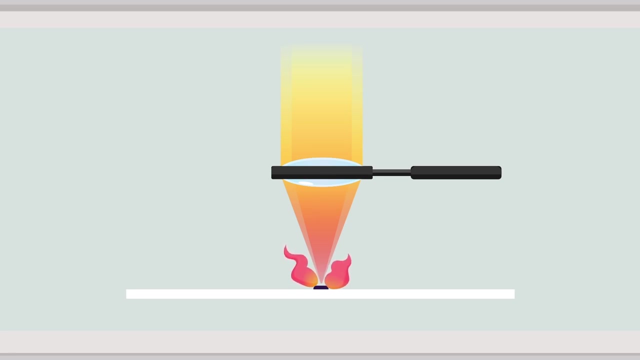 same amount of sunlight hits only a small area at low latitudes, but is spread over a large area at high latitudes. We have all experimented with lenses focusing pinpoints of light onto pieces of paper to make them burn. This experiment shows how the same amount of heat concentrated in a smaller area. 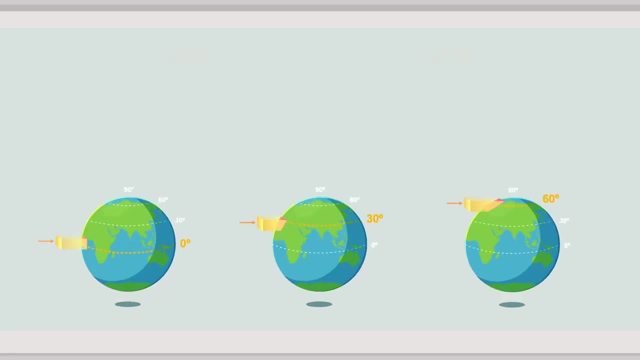 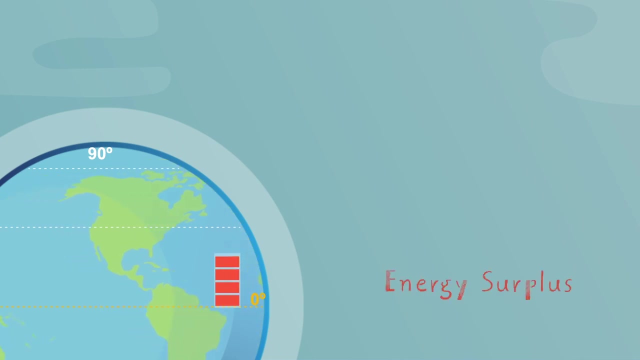 results in a higher temperature. The amount of energy received per unit of area is greater at low latitudes than at high latitudes, and this is why it is hotter in the tropics. At low latitudes, there is surplus energy because the 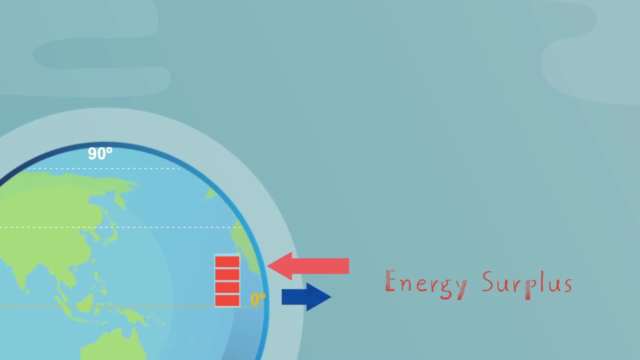 amount of heat radiated from the Sun is greater than the amount of energy radiated from the earth At high latitudes. there is an energy deficit because the earth gives out more energy than it receives from the Sun. This energy imbalance, caused by differences in energy received from. 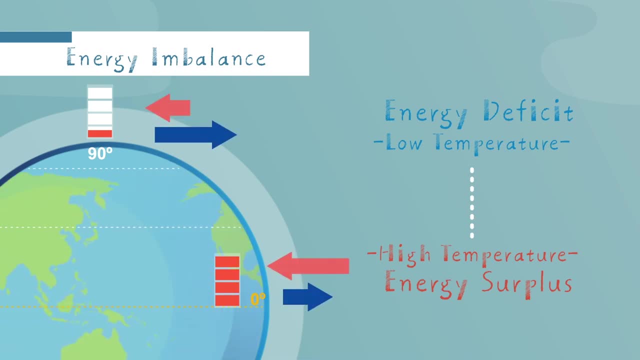 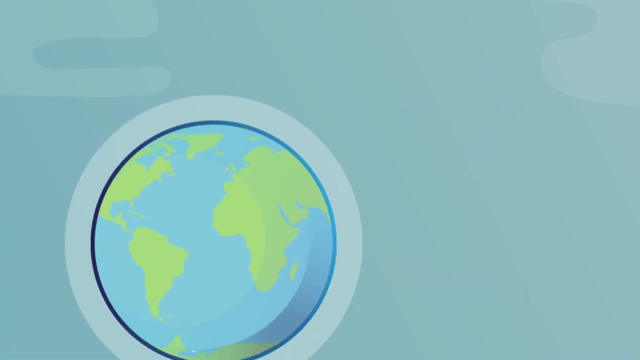 the Sun and emitted from the earth according to latitude, is one of the two causes of atmospheric general circulation. The other cause of atmospheric general circulation is the Coriolis effect or the Coriolis force. The Coriolis effect is a force created by the rotation of the earth that acts clockwise. 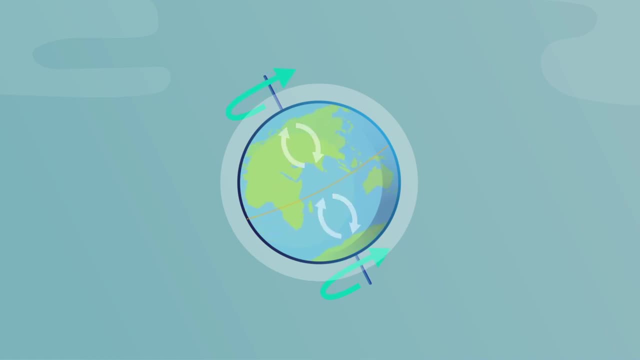 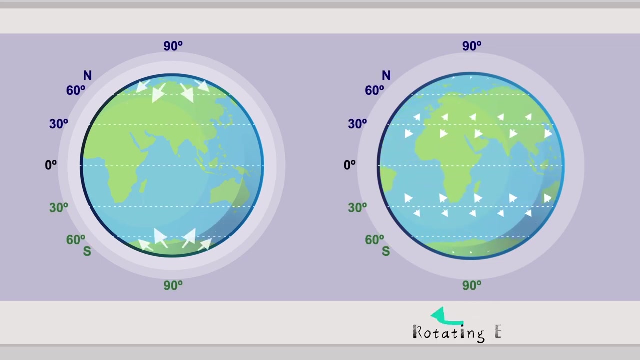 in the northern hemisphere and, counterclockwise, in the southern hemisphere. The Coriolis effect is not an actual force. It only appears to exist. To understand the Coriolis effect we need to look at atmospheric general circulation on the rotating earth and on a hypothetical stationary earth. 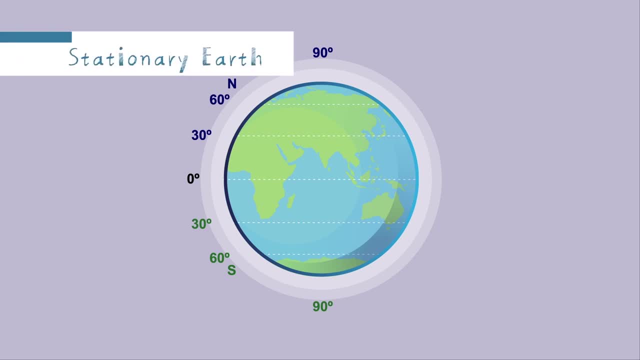 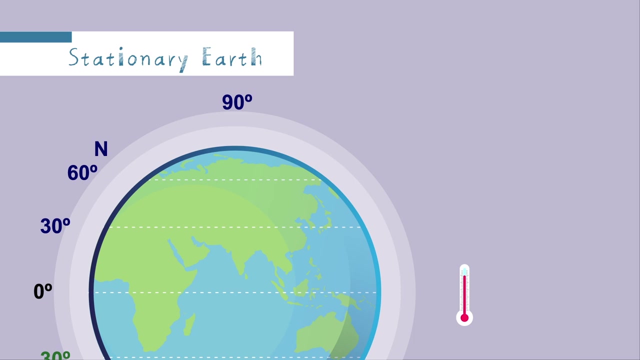 First, let's pretend that the earth is stationary and does not rotate. Warm air is lighter than cold air and has a strong tendency to rise. The air at the tropics is warm due to the high temperatures in the area and has a tendency to rise. 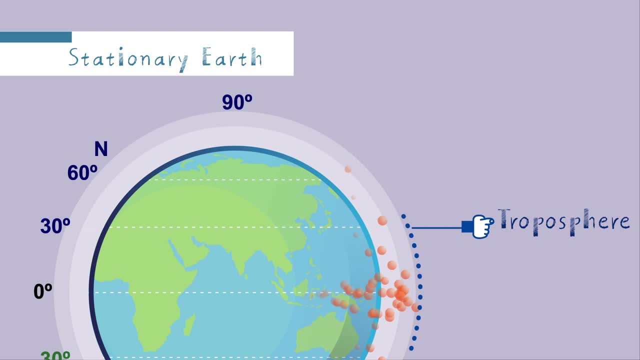 However, this air cannot rise above the troposphere, With nowhere else to go. the air spreads out horizontally and moves to higher latitudes. At higher latitudes the air is cooled, sinks down and travels back down to the tropics. 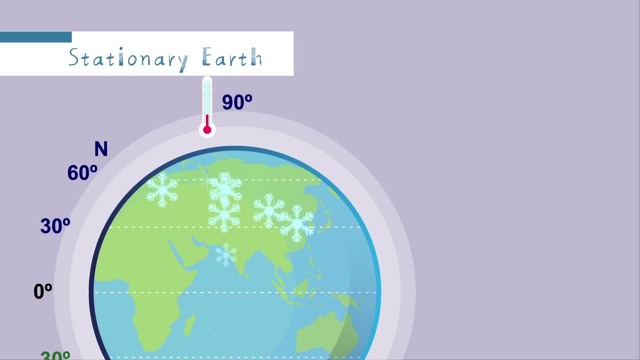 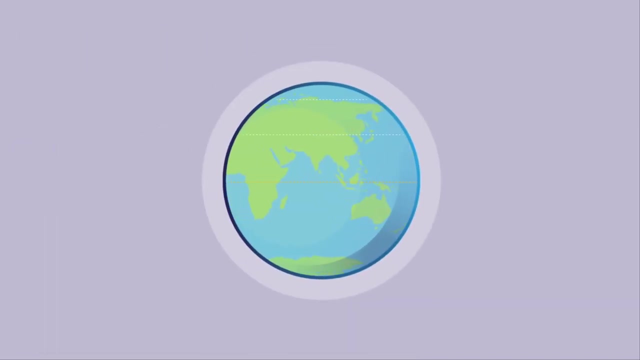 moving along the ground. Without the Coriolis effect caused by the earth's rotation, we would have only a single circulation cell, with only northerly winds blowing across the surface of the earth. So then, what happens on a rotating earth? 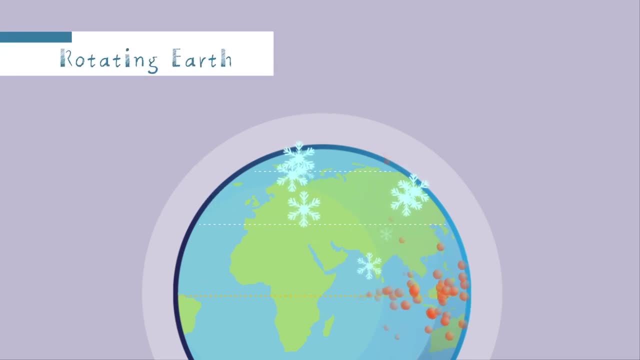 Here also. air rises in the tropics then falls back down at high latitudes. However, when the heated air in the tropics rises and the cold air falls back down to the tropics, the Coriolis effect causes the flow of air to bend to the right, creating 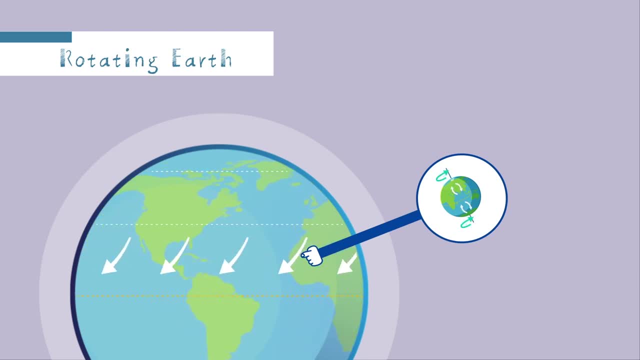 northerly winds. This is how the northerly trade winds are formed on the ground in the northern hemisphere. Due to the Coriolis effect, three circulation cells are formed in the atmosphere. These three circulation cells cause the trade winds, the westerlies and the polarity to 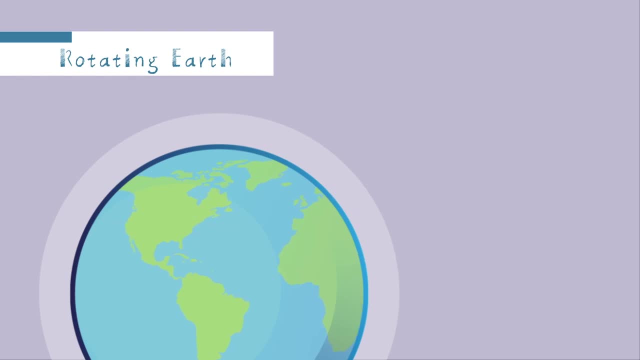 rise. The polarity of the Coriolis effect is the same as the polarity of the westerlies on the surface of the earth. Let's look now at the winds and atmospheric circulation at the latitudes of 30 degrees, 60 degrees and 90 degrees. 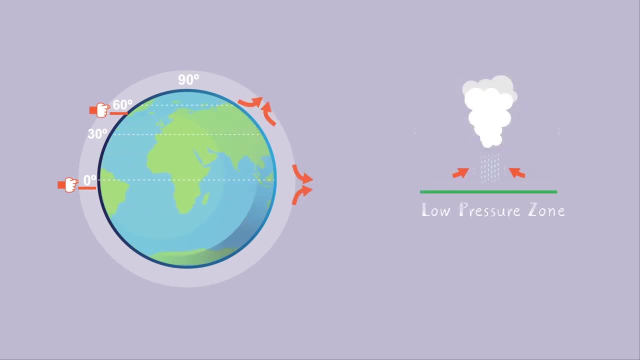 First, 0 degrees and 60 degrees latitude, are low-pressure zones with rising air currents. Here there is a large amount of precipitation. At 30 degrees and 90 degrees latitude are high-pressure zones with descending air currents. At 30 degrees latitude, Hadley circulation causes the trade winds on the earth's surface. 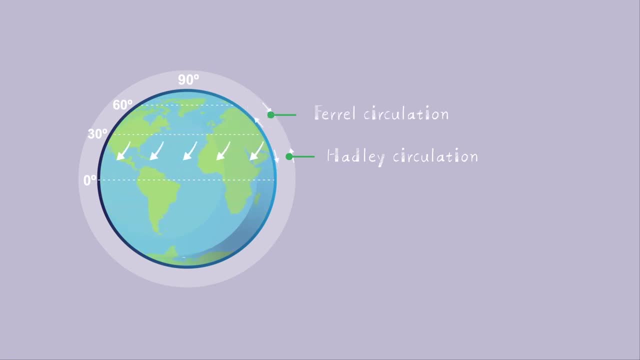 while at 30 degrees to 60 degrees latitude, Farrell circulation causes the westerlies. Lastly, at 60 degrees to 90 degrees latitude, polar circulation causes the polar easterlies. We mentioned before that the circulation of the atmosphere and seawater helps the earth. 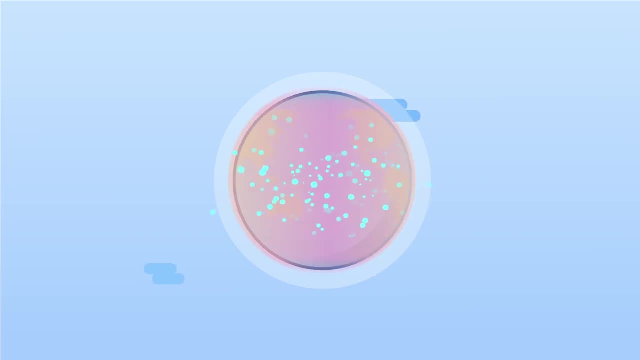 overcome latitudinal energy imbalances and maintain its constant temperatures. Now we will examine the circulation of ocean surface currents. Surface currents are horizontal flows of seawater that continue to flow in a certain direction, Like the circulation of the atmosphere. these surface currents transport heat from low latitudes. 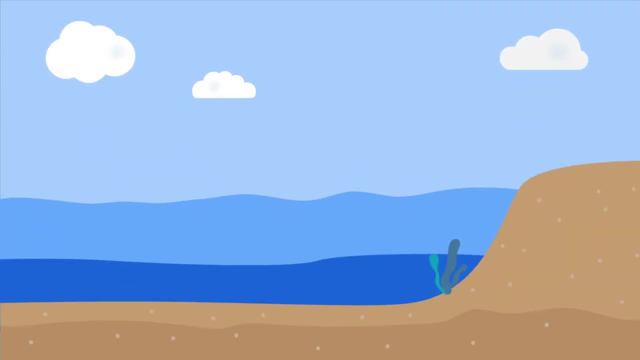 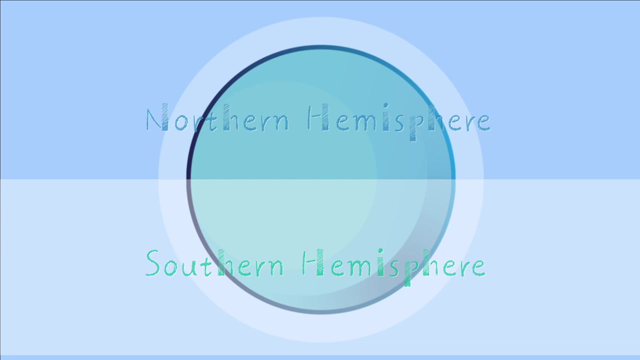 to high latitudes. Surface currents are caused by friction between the ocean surface and the winds that blow in a constant direction. due to atmospheric general circulation, Surface currents in the northern and southern hemispheres are different. In the northern hemisphere there are three kinds of circulation: tropical, subtropical. 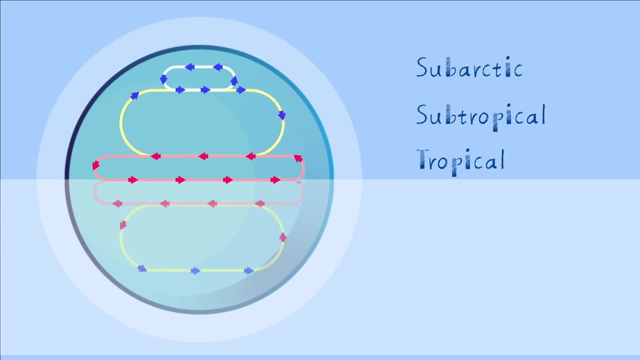 and subarctic. However, in the southern hemisphere there are only two types of circulation: tropical and subtropical. Tropical circulation occurs near the tropics, moving in a counterclockwise direction in the northern hemisphere and a clockwise direction in the southern hemisphere. 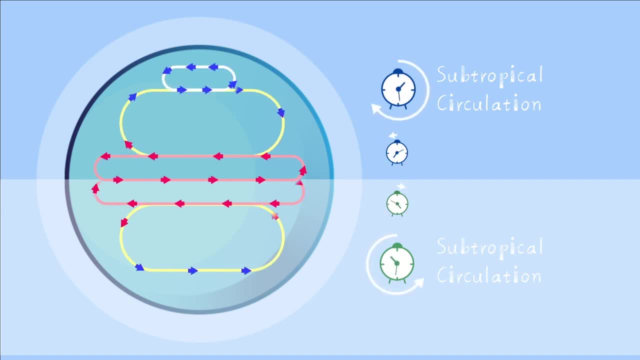 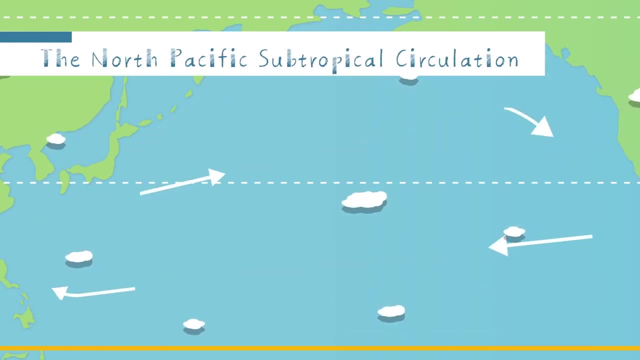 Subtropical circulation moves clockwise in the Northern Hemisphere and counterclockwise in the Southern Hemisphere. The most important type of circulation, the North Pacific Subtropical Circulation or gyre, can further be divided into the North Equatorial, Kuroshio, North Pacific and California currents. 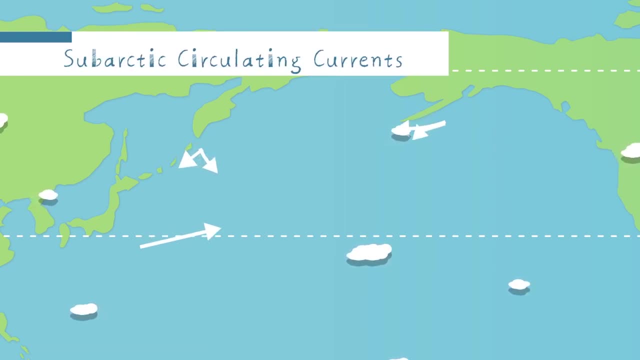 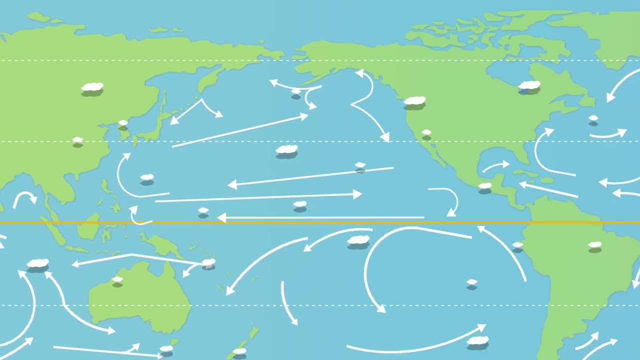 Examples of subarctic circulating currents found only in the Northern Hemisphere include the North Pacific Current, the Alaska Current and the Oyashio Current, also known as the Kuril Current. Why are there more types of circulation currents in the Northern Hemisphere than in the Southern? 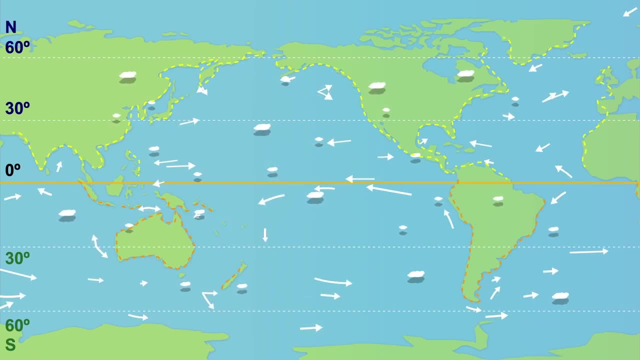 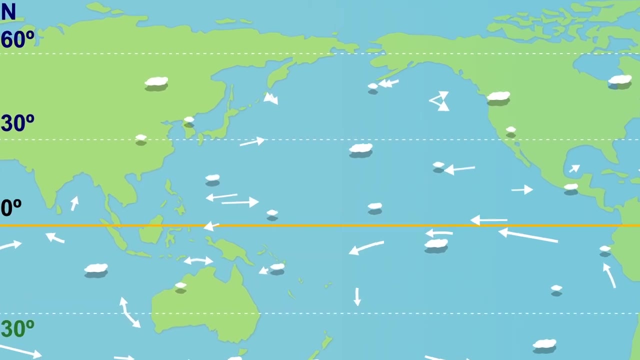 Hemisphere. The reason is because the Northern Hemisphere has more continents. More continents means that the currents are more broken up. Now let's look at the currents around Korea. However, before we do, let's talk a little more about warm currents and cold currents. 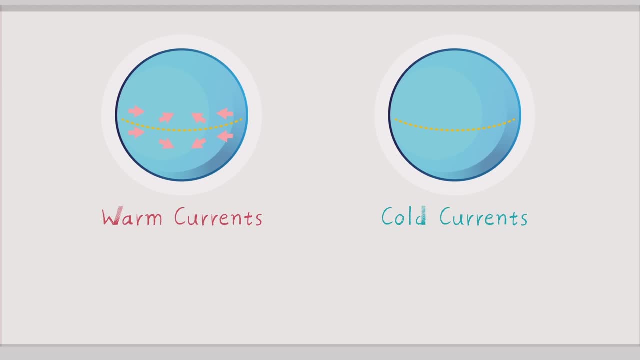 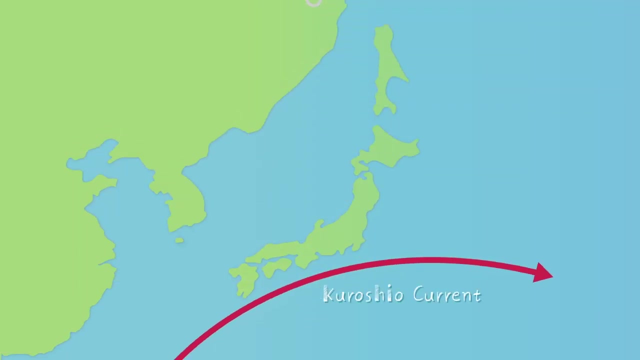 Warm currents are sea currents that move from low to high latitudes, while cold currents are those that move from high to low latitudes. Warm currents are warmer and have a higher salt content than cold currents. The warm current near Korea is the Kuroshio Current. 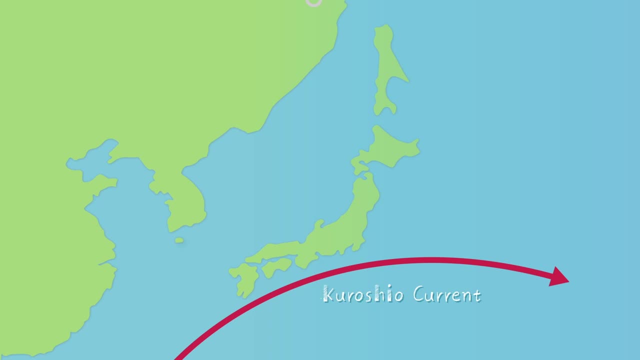 The Kuroshio Current, which is part of the North Subtropical Gyre, has the biggest impact on Korea. The Kuroshio Current results in the Yellow Sea Warm Current, the East Korea Warm Current and the Tsushima Warm Current. 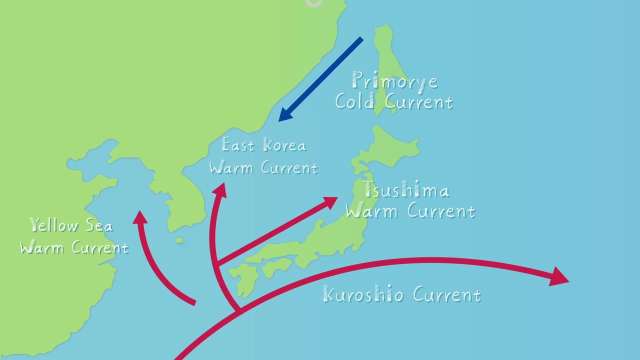 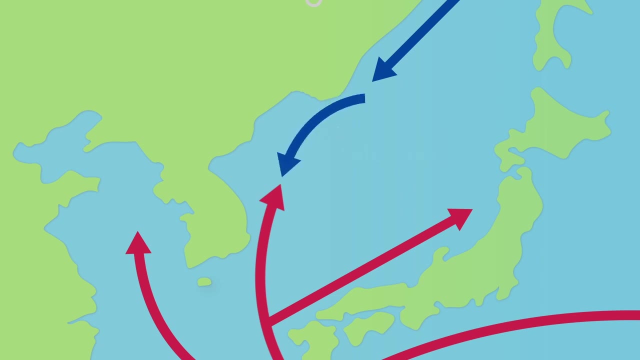 The cold current near Korea is the Primorye Cold Current. The North Korean Cold Current is part of the Primorye Cold Current and flows southward toward Korea. This creates a boundary line in the East Sea where warm currents and cold current meets. 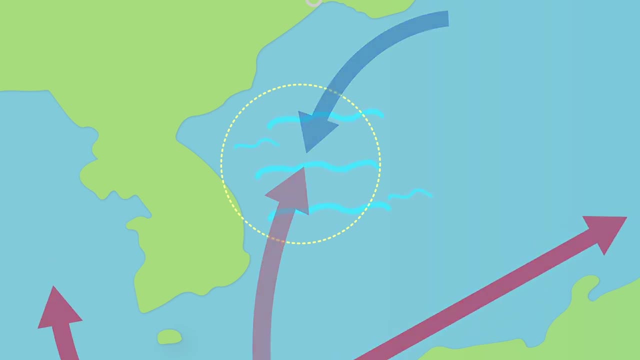 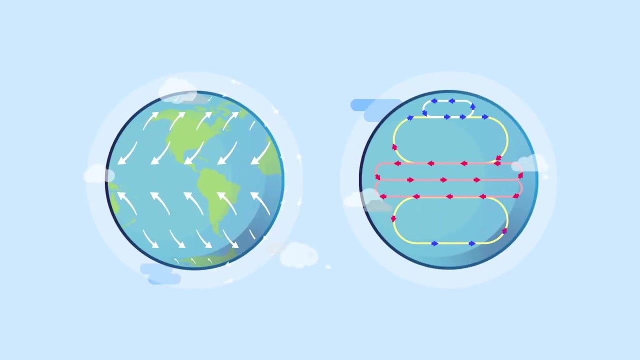 and this is the reason why the Korean Peninsula is surrounded by such rich fishing grounds. Today we studied the atmospheric general circulation of the North Subtropical Gyre. It's amazing to think about how the air and water on this vast earth are constantly moving. 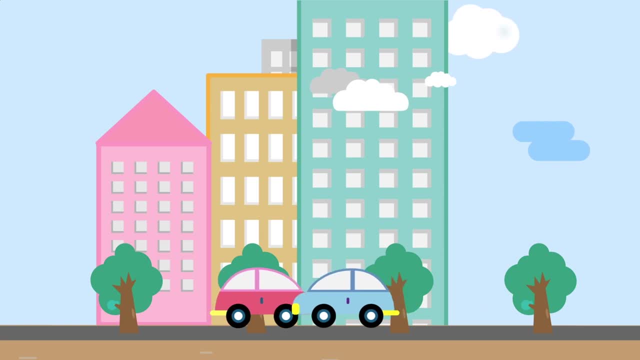 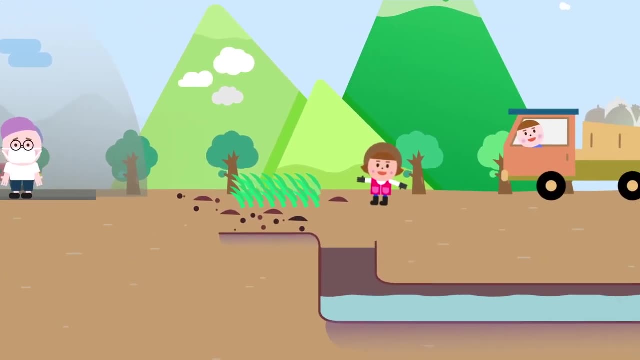 This might be a good time to bring up the issue of environmental pollution. Atmospheric pollutants such as fine dust and smog, water pollutants from garbage on land and oil leaks and soil, pollutants from chemical fertilizers, food waste and household waste are also being circulated in the atmosphere and by the oceanic surface currents. 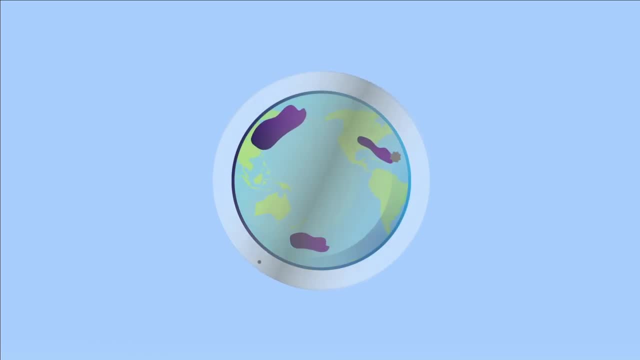 This is a good time to bring up the issue of environmental pollution: Atmospheric pollutants such as fine dust and smog, water pollutants from garbage on land and oil leaks, and soil pollutants from chemical fertilizers, food waste and soil pollutants from chemical fertilizers, food waste and soil pollutants are also being circulated. 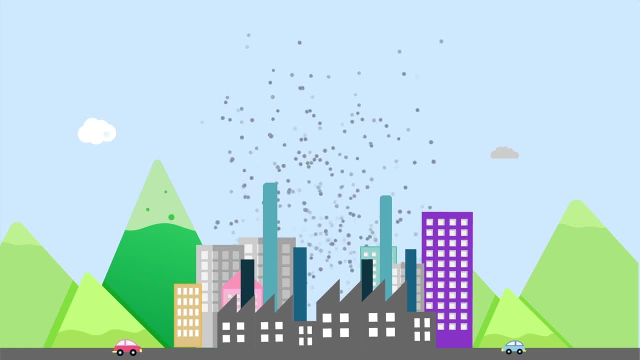 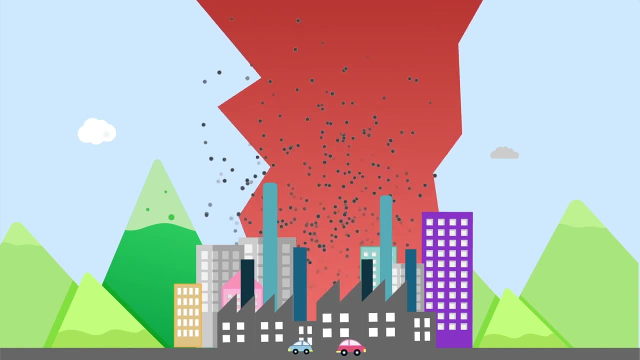 in the atmosphere and by the oceanic surface currents. It's a terrifying thought, isn't it? Next time, we will discuss global warming and the destruction of the ozone layer, a man-made phenomena caused by scientific and technological developments made for the sake.